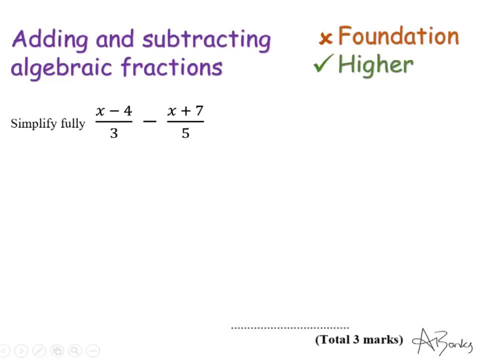 when we don't have algebra on the denominators, here we only have integers, it is generally easier. So as I would with adding and subtracting fractions, the first thing I'm going to do is find a common denominator. So here I have 3 and 5 on the denominators. My lowest common multiple is going to be 15. So putting a 15 on the bottom. Now the first fraction is going to be 15. So I'm going to put 15 on the bottom. So I'm going to go from the 3 on the denominator to the 15. I am multiplying by 5. So I need 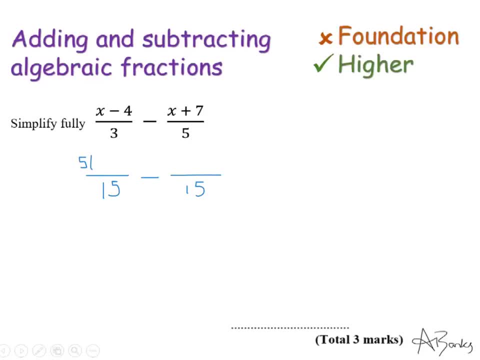 to multiply the numerator by 5 as well. And for now I'm just going to leave it in brackets. 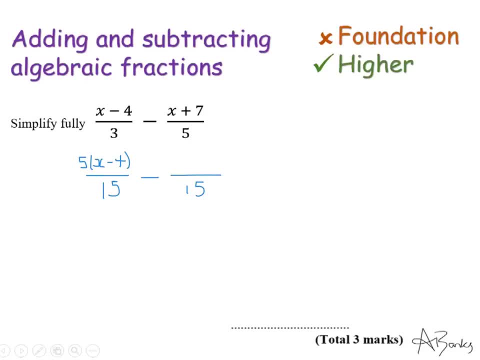 So I'm going to do all of that multiplied by 5. And then on my second fraction I multiply everything by 3. So that's my first step and that will get me some marks. Now I'm going to expand the numerators. So this is 5x minus 20 over 15 minus 3x plus 21 over 15. Now I've just got to write these as one fraction. And I can do this now that my denominators are the same. So I have 5x minus 20. Minus 3x minus 21. Just be careful at this step here. If it was 3x minus 21 in the numerator that would make it a double negative and I would have minus 3x plus 21. So just be careful of that step. And this is all over 15. Now to simplify my numerator, 5x minus 3x is 2x. And minus 20 minus 21 is minus 41. 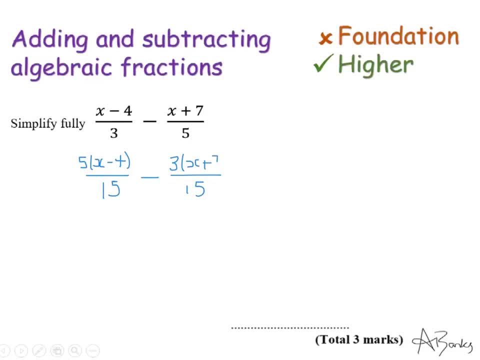 everything by 3.. So that's my first step, and that will get me some marks. Now I'm going to expand the numerators. So this is 5x minus 20 over 15, minus 3x plus 21 over 15.. Now I've just got to write these: 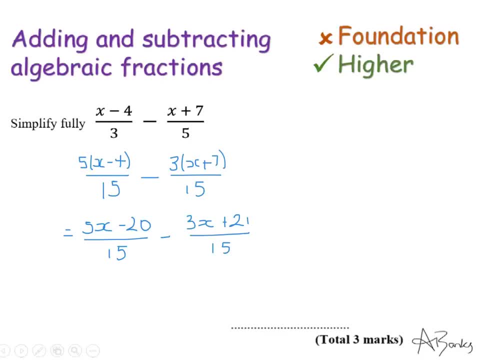 as one fraction, And I can do this now that my denominators are the same. So I have 5x minus 20.. Minus 3x minus 21.. Just be careful at this step here. If it was 3x minus 21 in the numerator, 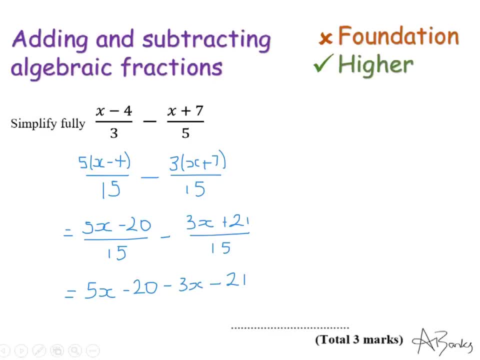 that would make it a double negative and I would have minus 3x plus 21.. So just be careful of that step. And this is all over 15.. Now to simplify my numerator: 5x minus 3x is 2x. 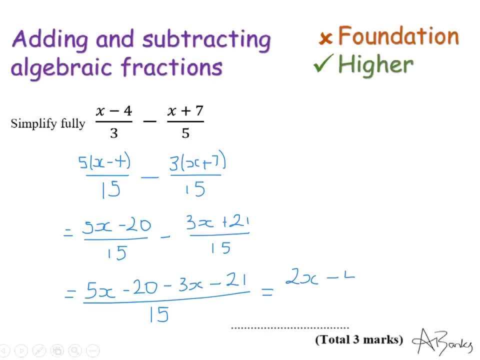 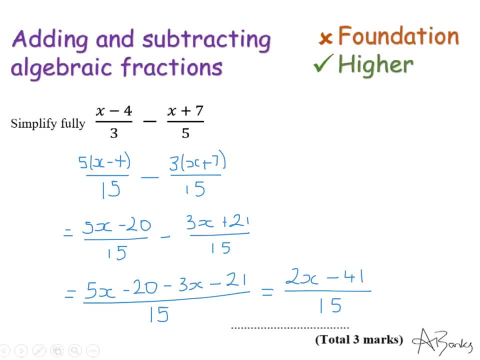 by 5.. So I'm going to do all of that multiplied by 5.. So I'm going to do all of that multiplied. no integer apart from 1 that divides 2,, 41 and 15.. That's my final answer. 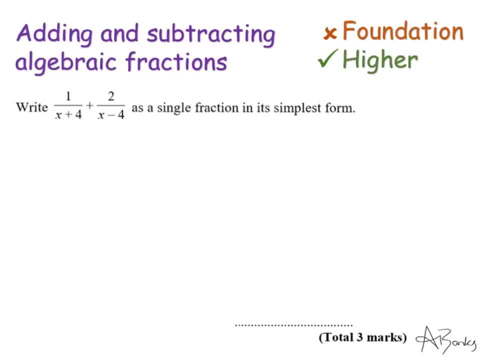 Here's a slightly more tricky example, because this time I have algebra on the denominators of my fractions, So I need to find some common multiple of x plus 4 and x minus 4.. Now the simplest way to do this: as we do with adding fractions, we could always multiply the denominators. 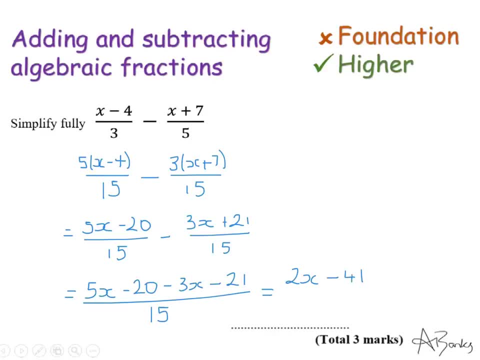 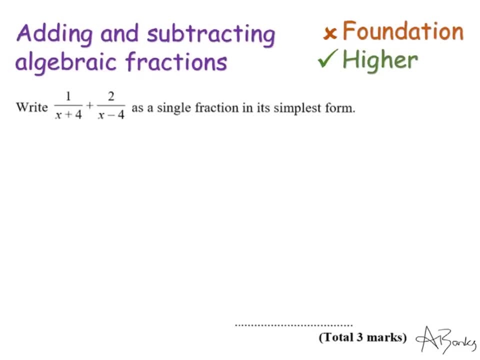 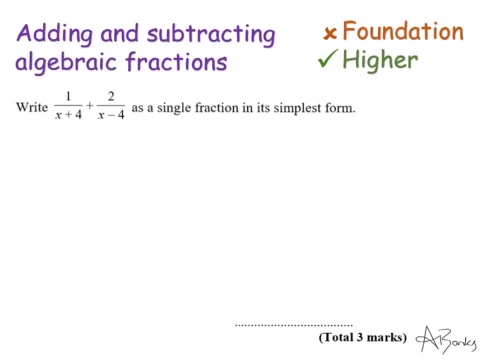 denominators of my fractions so I need to find some common multiple of x plus 4 and x minus 4 now the simplest way to do this as we do with adding fractions we could always multiply the denominators together so if I had a denominator of 6 and 8 I know for definite that 48 would work as a common denominator it might not be the best option but it certainly works and with algebra that's the only option we have so my first fraction I'm going to put my denominator x plus 4 and I'm going to put in double brackets x minus 4 now I've multiplied this fraction by x minus 4 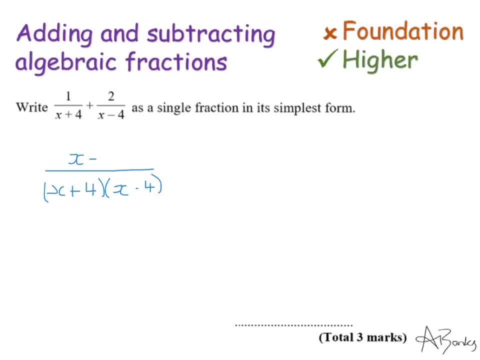 so my top I have to multiply by x minus 4 as well my second fraction I'm going to put the same denominator in the same order this one has been multiplied by x plus 4 so I'm going to multiply my numerator by x plus 4 now as before we just need to do a little bit of tidying up with this so the first thing I can do here is expand this bracket on the top so leaving the first fraction as it is 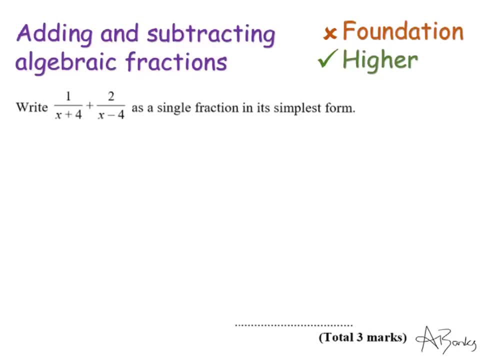 together. So if I had a denominator of 6 and 8, I know for definite that 48 would work as a common denominator. It might not be the best option but it certainly works And with algebra that's the only option we have. So my first fraction. I'm going to put my 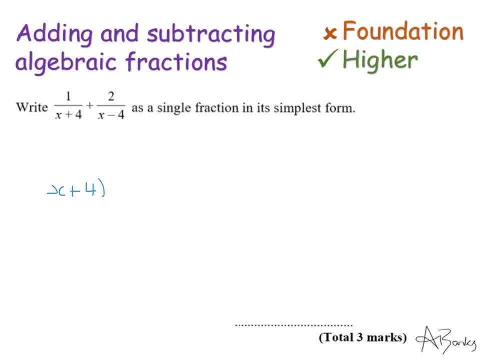 denominator x plus 4, and I'm going to put it in double brackets: x minus 4.. Now, I'm going to put my denominator x plus 4, and I'm going to put it in double brackets: x minus 4.. Now I'm going to put my denominator x plus 4, and I'm going to put it in double brackets. 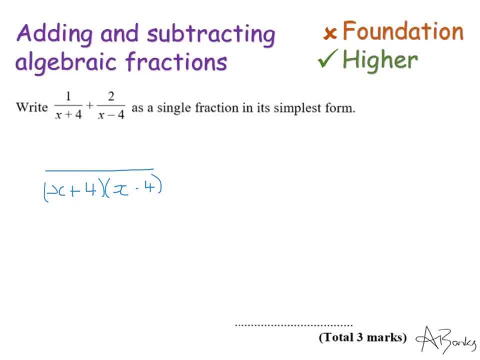 x minus 4.. Now I've multiplied this fraction by x minus 4.. So my top: I have to multiply by x minus 4 as well. My second fraction- I'm going to put the same denominator in the same order. This one has been multiplied by x plus 4, so I'm going to multiply my numerator. 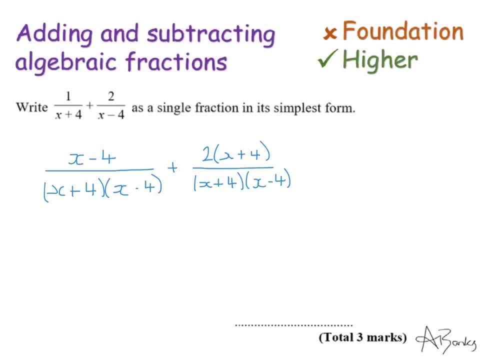 by x plus 4.. Now, as before, we just need to do a little bit of tidying up with this. So the first thing I can do here is expand this bracket on the top, So leaving the first fraction as it is, And my second fraction is going to become 2x plus 8 and the same denominator. Of course, you don't have 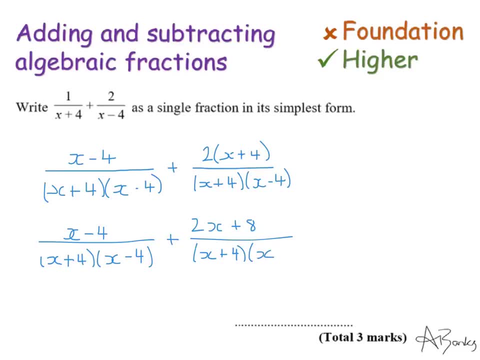 to do this step of working out. You could have worked out that it was 2x plus 8 on the numerator straight away. I'm just trying to show you every step of working out here, So my final answer here is going to be I: 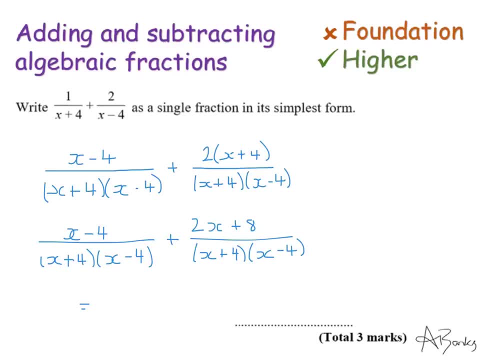 Have an x minus 4 and a 2x plus 8 on the numerators, so that's 3x plus 4. All over Now the denominator here. you can leave it as it is and that will still get you full marks. So I'm going to leave it as x plus 4. 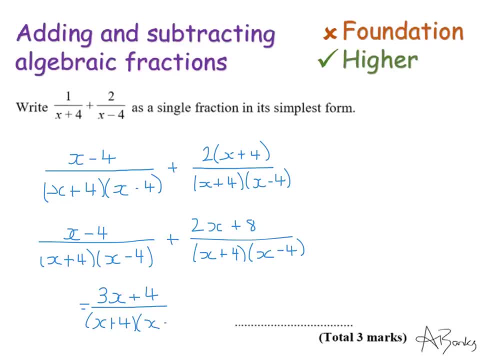 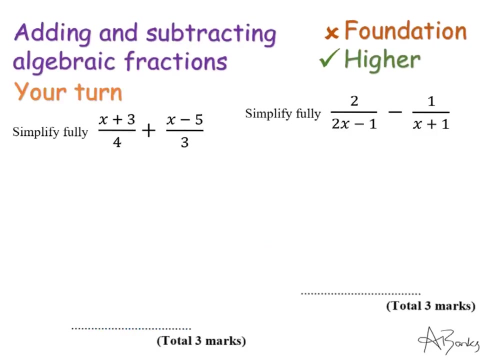 x minus 4. There's no need to create extra work for yourself there figuring that out, Unless the question Specifies that it wants the answer given in a certain form, and this one doesn't. it just say simplest form, So this is fine for full marks. Here's two questions for you to try. pause the video and then unpause when you're ready to see the solutions.